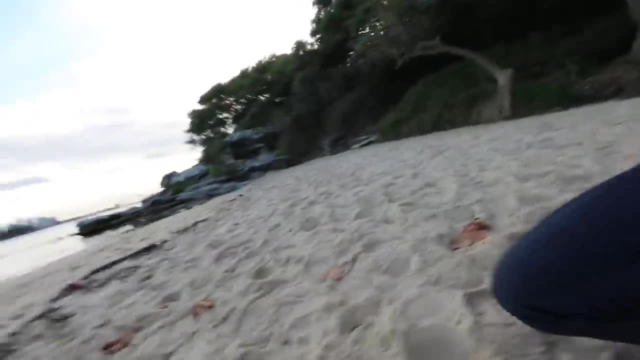 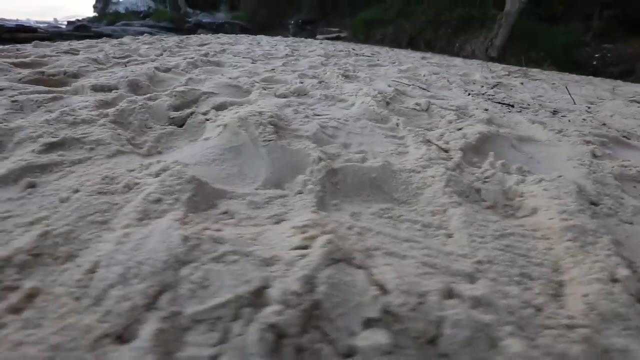 So the beach here has these undulations in it which represent the fluctuations in the gluon field. But you have to imagine this beach sort of rippling and these bumps coming and going. Now that's really important because to get rid of those fluctuations actually takes energy. 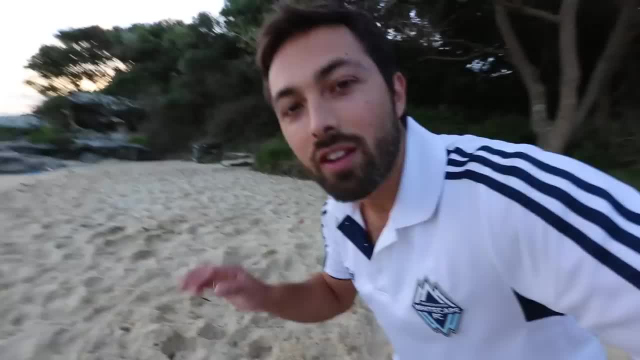 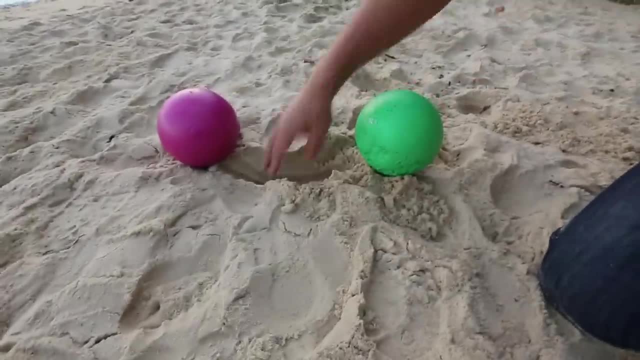 and this is an important part of binding the quarks together. The existence of quarks actually suppresses the gluon fluctuations and creates what's called a flux tube, an area where there is really nothing in the vacuum, and that's in between this quark and the anti-quark. 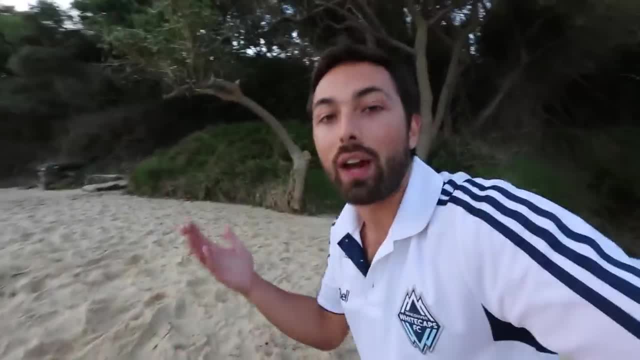 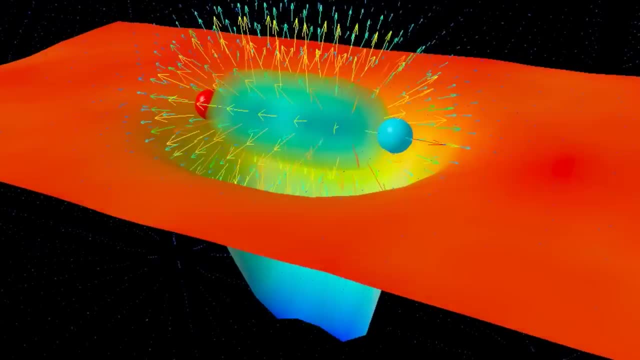 and that pairs them up and creates what's called a meson, the quark-anti-quark pair. What's interesting about the flux tube is that as these quarks become more separated, the flux tube remains the same diameter and the same sort of depth of suppression of the field. which means that the force doesn't actually increase. It's not like a spring, It's not like an elastic band. The force is the same. that is pulling these quarks back together, But you are putting more work in as you move these quarks and anti-quarks further apart. 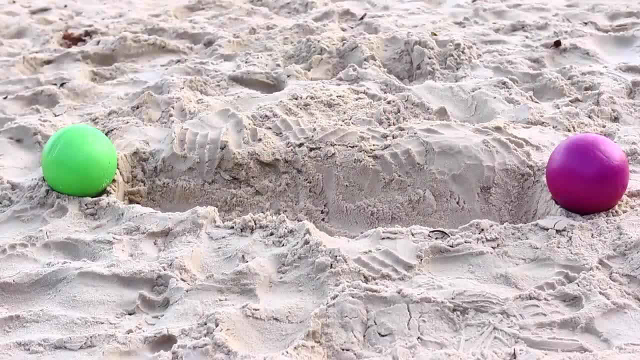 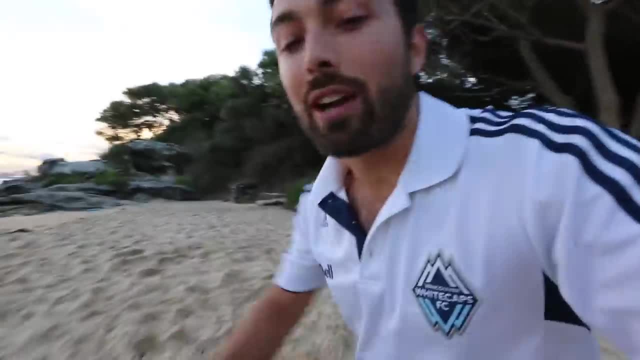 And so for a time, people thought: well, these quarks are always going to be confined, however far you move them. You're just going to get a really long flux tube. But what actually happens is that you put in enough energy that you can actually create a quark-anti-quark pair. 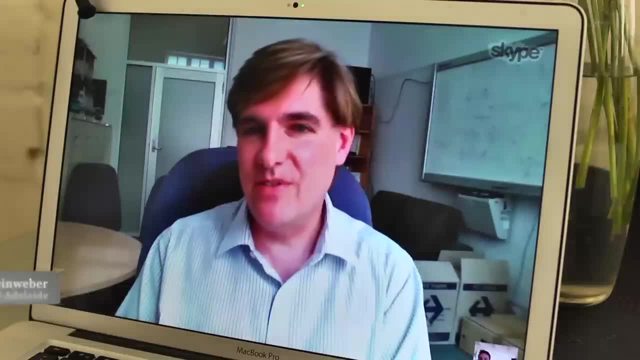 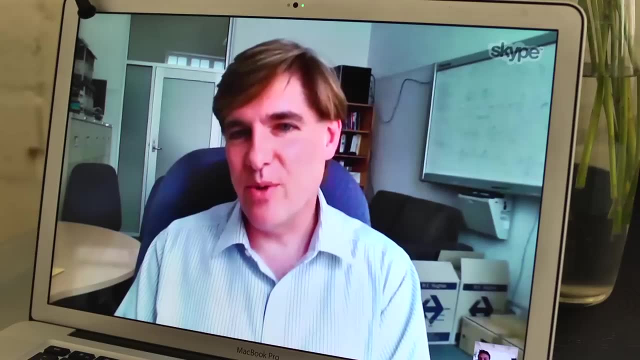 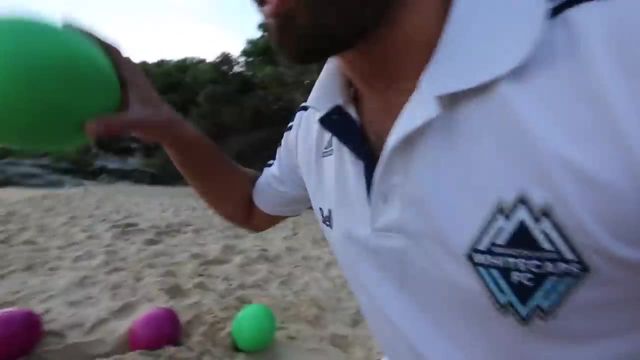 Nevertheless, the quarks are still confined. You can never see an individual quark because if you try to pull it out, you put so much energy into the situation that another quark-anti-quark pair will be created. Now to form a proton. we're going to need an up quark, another up quark and a down quark. 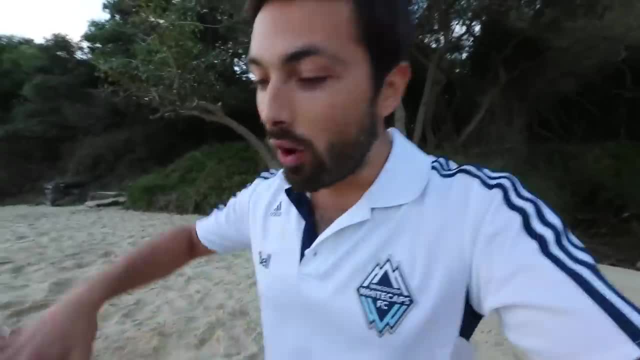 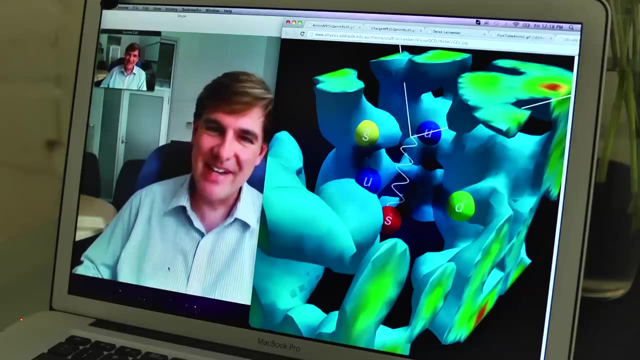 Now the standard model of a proton that you've probably seen involves these quarks bounded together by little gluon springs that go between them. We know that that picture is totally wrong. now, Even in the best sense, you might have hoped that you would see flux tubes around the edge of the triangle. 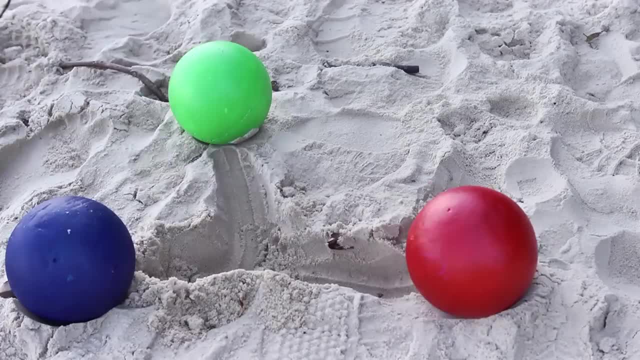 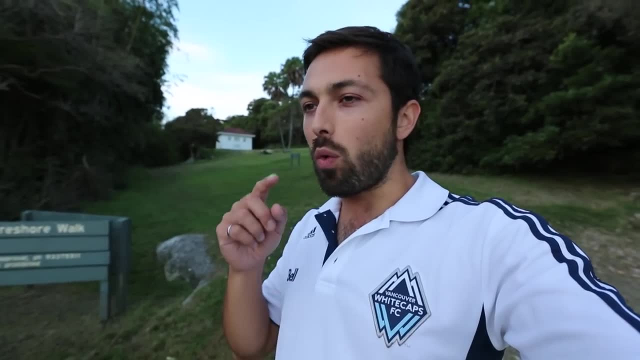 But we know that in fact they don't do that- That you get these Y-shaped flux tubes. The crazy thing about a proton is that there may be more than three quarks there. You see, you can have additional quark-anti-quark pairs, pop in and out of existence. 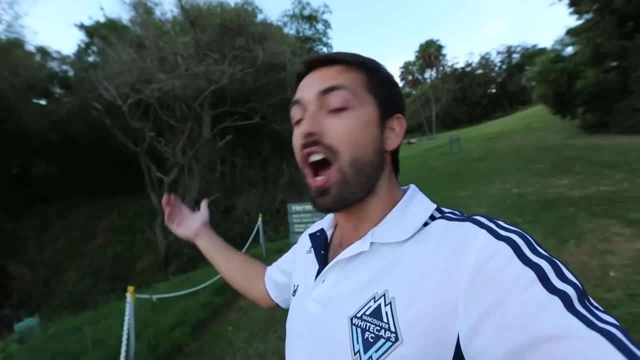 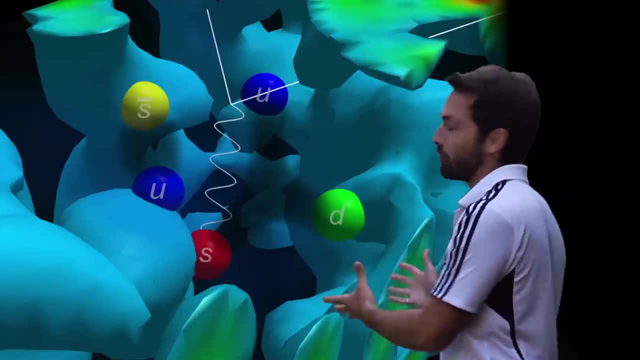 So at any given time there could be five or seven or nine. any odd number of quarks could make up a proton. So this is what a proton actually looks like. You can see that the quarks like to sit on those lumps in the gluon field. 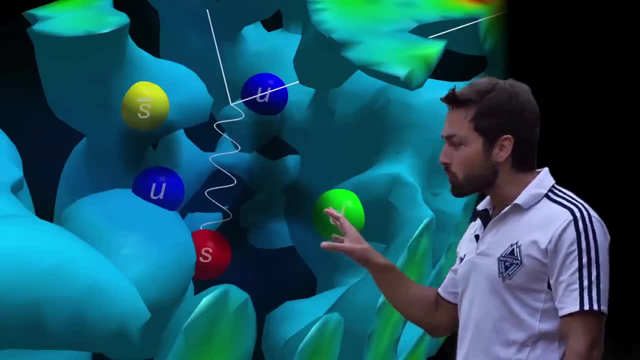 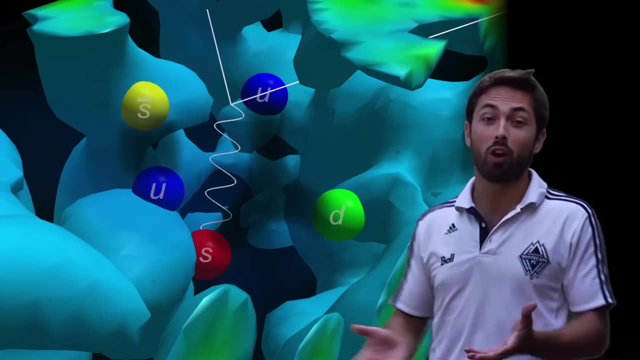 And you can see the two up quarks and a down quark. but there's also a strange quark and an anti-strange quark, Which is strange because you don't normally think of these quarks being inside a proton, but they can be at any particular point in time. 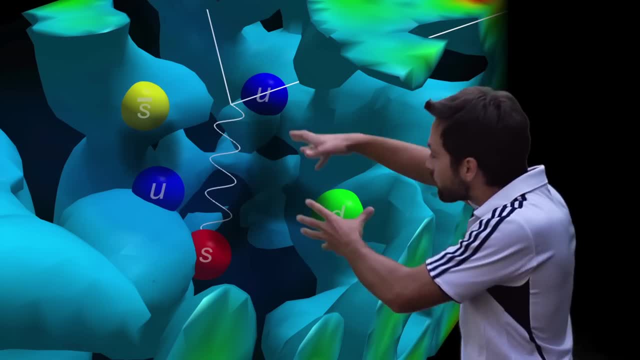 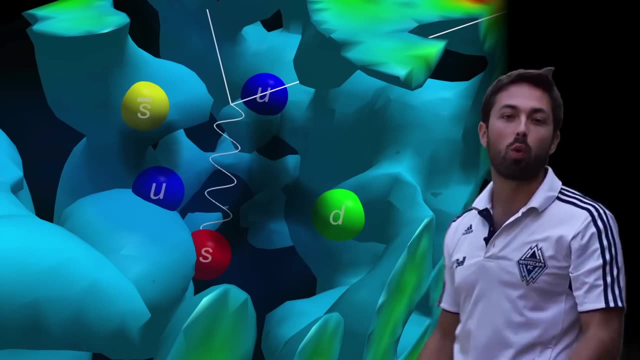 You can also see that these quarks have cleared out the vacuum And you can see there's kind of these flux tubes which are the areas where the gluon field has been suppressed, And that's really what's binding these quarks together. That's the strong force that binds quarks into the heart of the proton. It is intrinsically related to the fact that clearing out those fluctuations has more energy than where they are. That's right. It costs energy to clear the vacuum. So where is the mass of the proton really coming from? Well, of course the constituent quarks do interact with the Higgs field and that gives them a small amount of mass. But if you add up the mass of all the quarks in the proton, it would only account for about 1% of its total mass. 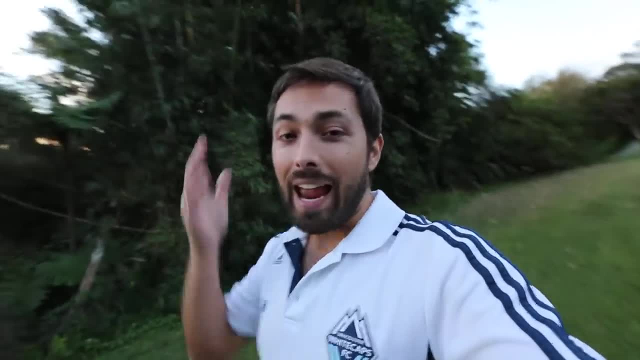 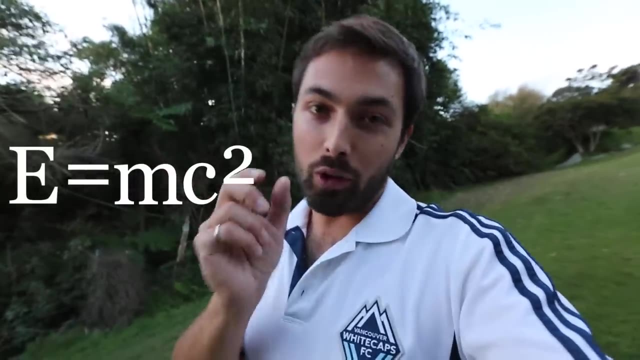 So where's the rest of the mass coming from? The answer is energy. You know Einstein's famous equation: E equals MC squared. Well, that says we got a lot of energy for just a little bit of mass. But if you rearrange the equation, 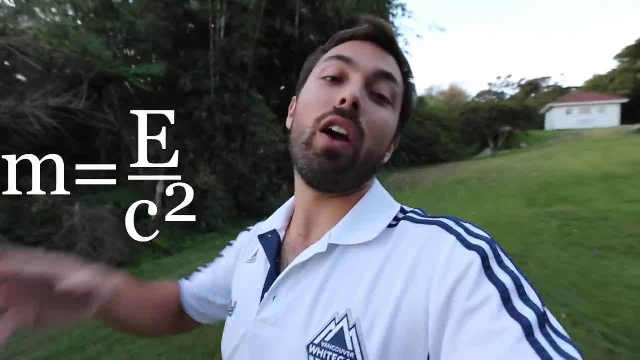 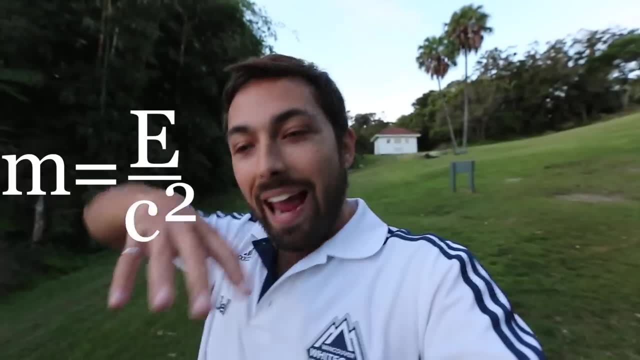 you can see that we can get an amount of mass if there is lots of energy there, And that is really where most of the mass of the proton is coming from. It's from the fact that there are these energy fluctuations in the gluon field. 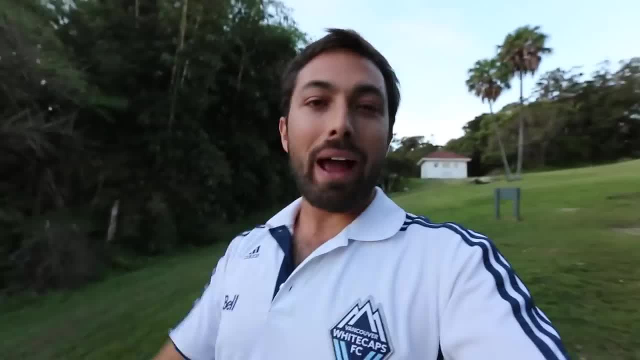 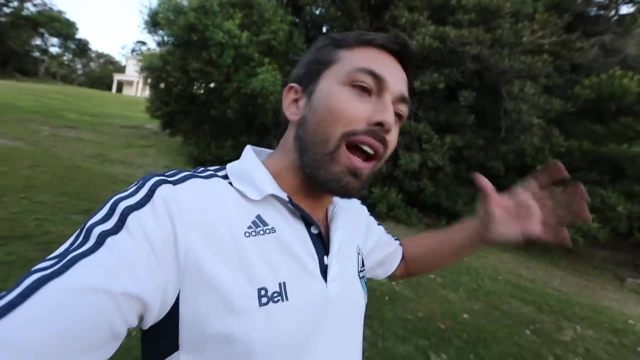 and the quarks are interacting with those gluons. That is where your mass is coming from. It's coming from the energy that's in there. You know Einstein talked about. well, if I had a hot cup of tea, it would actually have a slightly greater mass than the same cup of tea when cold. 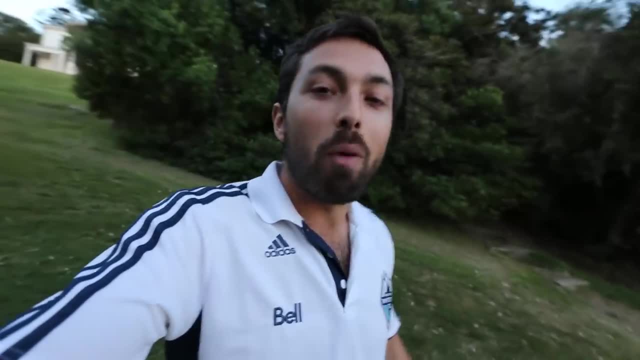 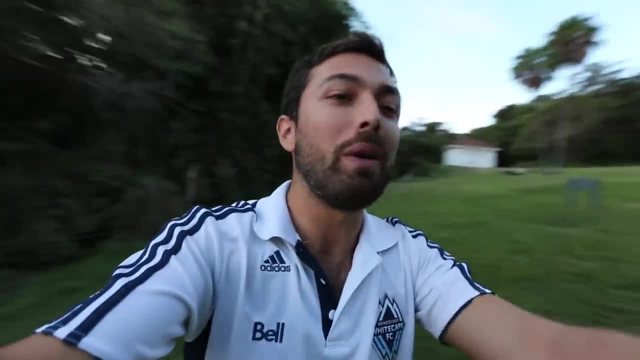 And he was right. I mean, you can't measure it with a cup of tea, But most of your mass you owe to E, equals MC squared. You owe to the fact that your mass is packed with energy because of the interactions between the quarks and these gluon fluctuations in that gluon field. 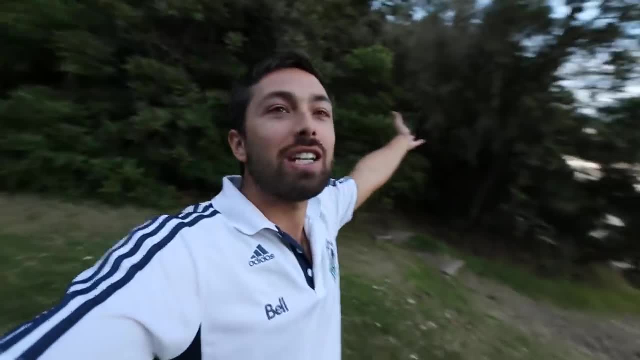 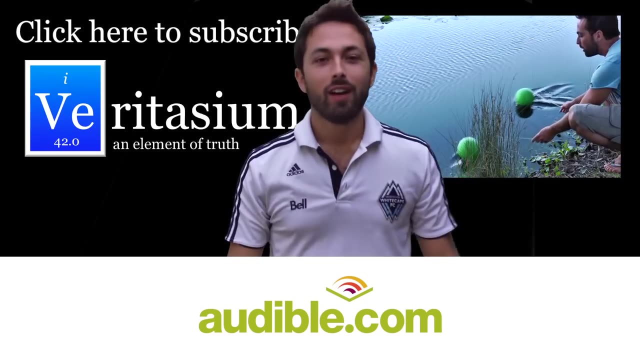 I think it's extraordinary, because what we think of as ordinarily empty space, you know that- turns out to be the thing that gives us all most of our mass. I really want to thank Audiblecom for supporting this episode of Veritasium.